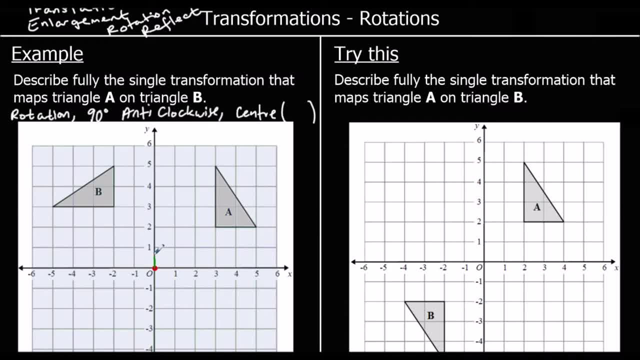 to move shape A onto shape B B. so let's draw a north line here. I'll go around shape a. so if I hold the tracing paper at zero, zero at the center, will shape a go on to shape B. so I'm going to turn it 90 degrees anti-clockwise and shape a goes on to. 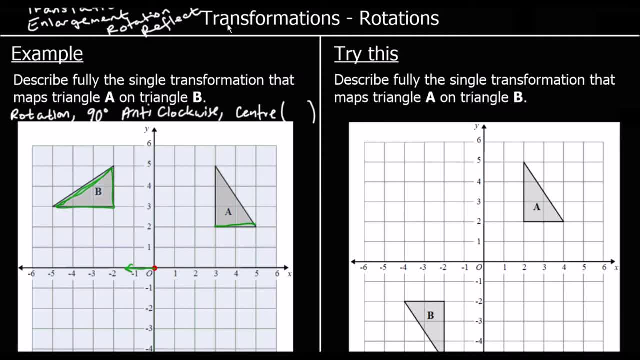 shape B. so it's Center is at zero, the origin Center at the origin. so it's a rotation 90 degrees anti-clockwise, or we could say we could go 270 degrees clockwise. it's the same thing. so 90 degrees anti-clockwise with the center of the origin, and that is all the information. 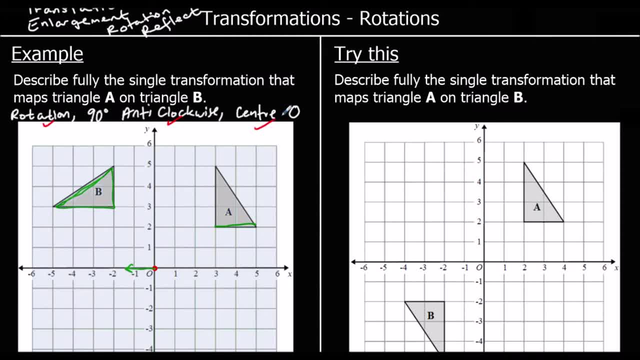 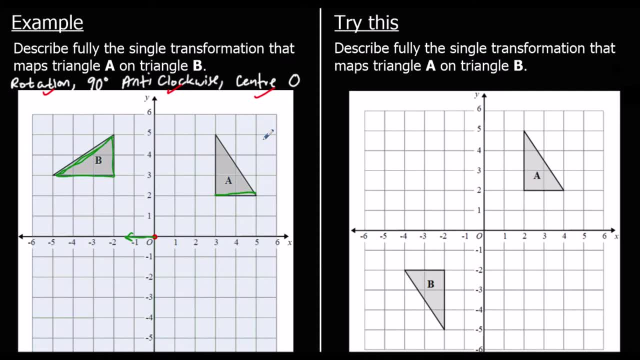 that we need to give these three parts to describe a rotation. so here's one for you to try so describe the transformation that maps triangle a onto triangle B. so again, it is a rotation. so the first bit of information we need is the rotation. so the first bit of information we need is the rotation. so 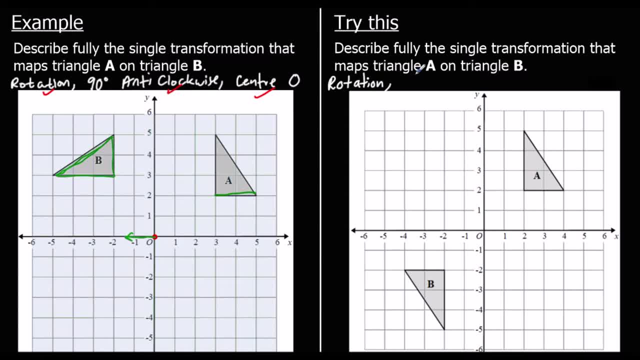 is rotation. how far has it turned? so this is 180 degrees, it's a whole, half a turn, 180 degrees. we don't have to give clockwise or anti-clockwise, because it would be the same both ways. and what's the center? so where do we have to hold? 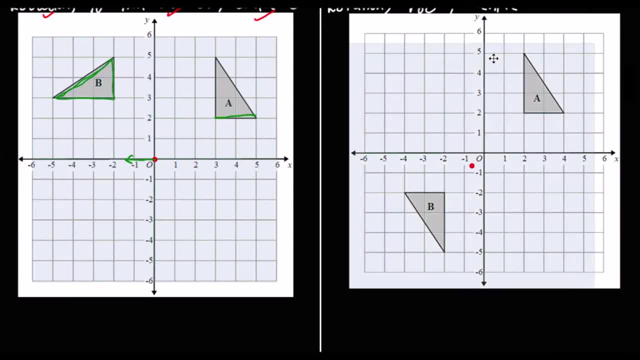 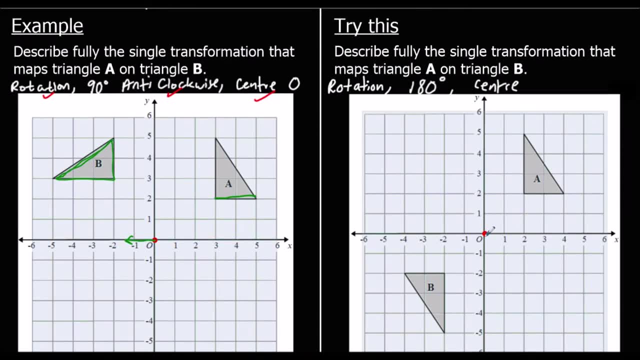 the tracing paper. so if we grab some tracing paper now, try it at the origin again. so I'm going to draw a line going up and I'm going to draw a round shape, a. so if I rotate this shape, if I rotate this tracing paper 180 degrees, so the arrow. 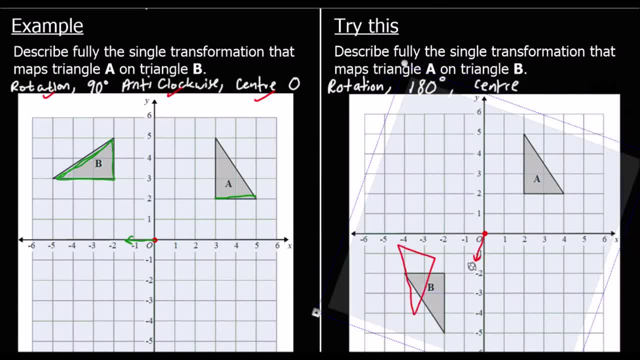 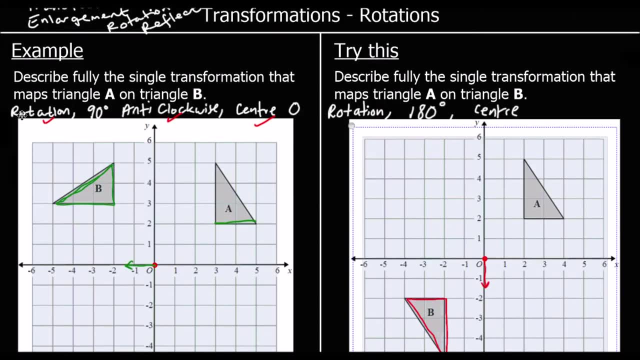 would be going down. will shape a go to shape B? yes, it will. so you can see it's 180 degrees, 180 degrees and the center is again at the origin. it's a rotation 180 degrees, center at the origin. and another question: describe fully the single. 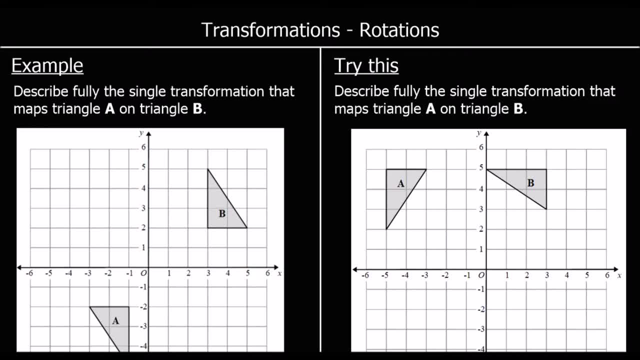 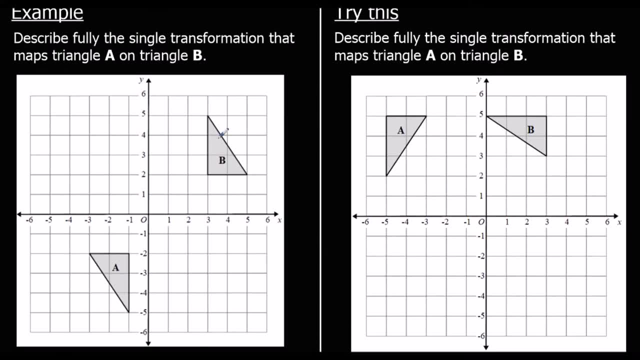 transformation that maps triangle a on to triangle B. so triangle a is down here, triangle a is down here, and again it's going to be a rotation, so we're going to create two segments. right, we're going to click the 3D via anchor method. it's. 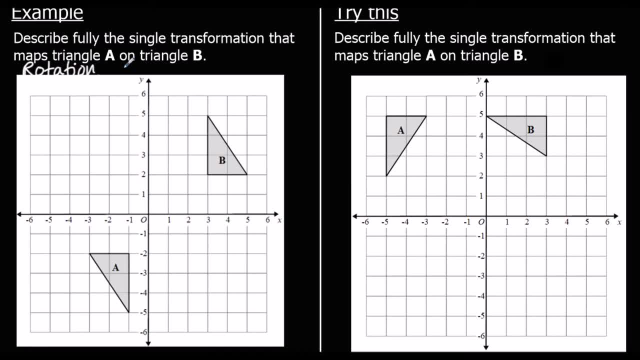 going to be a rotation and this is 180 degrees rotation. so it's rotation, 180 degrees. we don't have to say clockwise or anti-clockwise, because it would be the same thing both ways around, and we just need to know the center. so where do 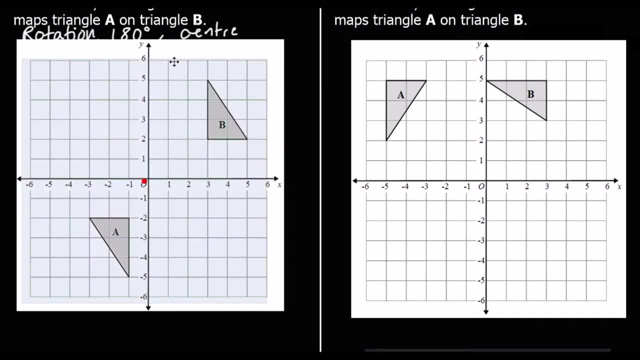 we hold the tracing paper, so let's grab the tracing paper and I'll try it at the origin again. so I'm going to draw a line going north and I'm going to draw a round shape a. so if I rotate this 180 degrees, will it go on to shape B? no, it won't. so the tracing 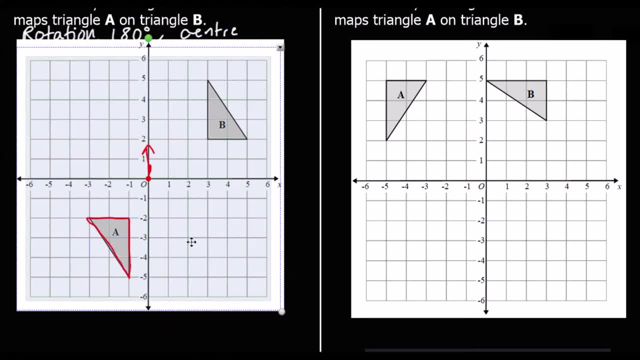 paper is being held in the wrong place so I'm going to move it. so, if I try, from one zero. so now I'm going to hold my tracing paper at one zero and rotate it and we can see it goes on to shape B, so the center this time is at one zero. 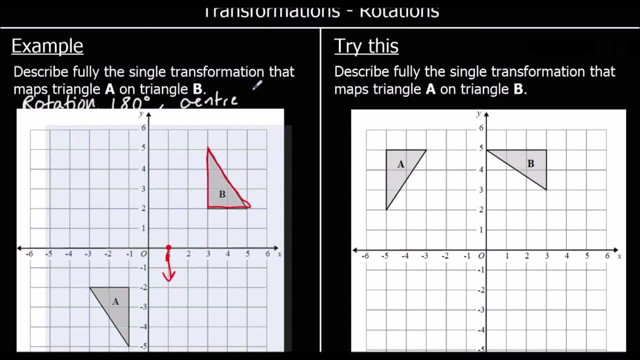 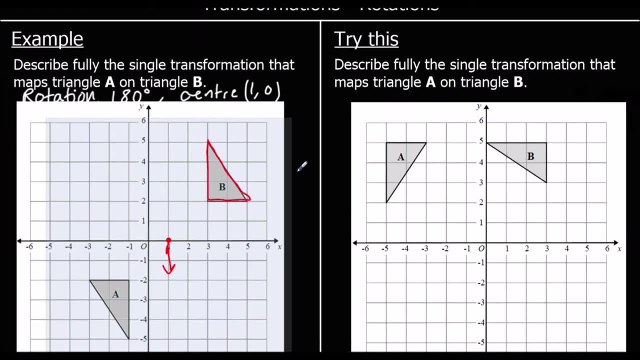 so center, one zero and one for you to try so describe the transformation that maps triangle a onto triangle B, so we can again see it's a rotation and it's gone 90 degrees clockwise. but where do we hold the tracing paper? where is the center? so let's try and figure that out. so let's get the tracing paper. 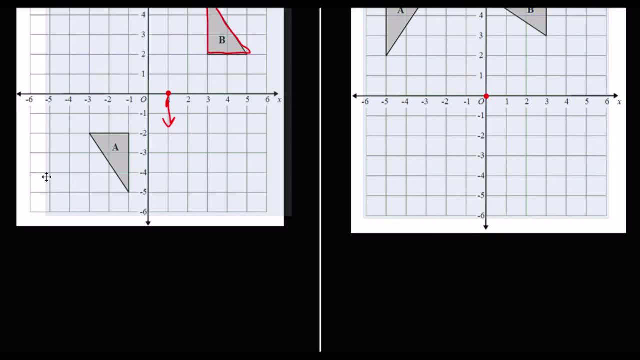 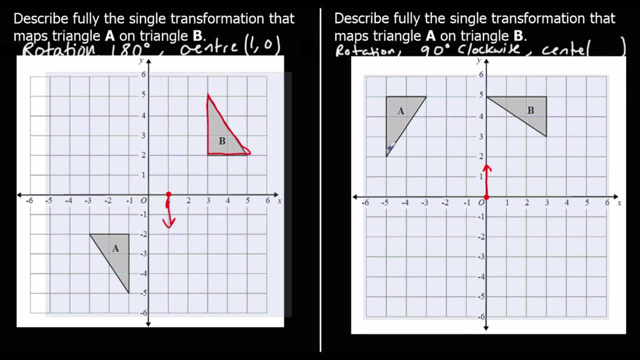 you. so I'll draw a line going up and draw around shape a. so if I held the tracing paper at the origin, there's the shape. go to the right place. no, it's not. it's not in the right place, it's gone too far to the right. so 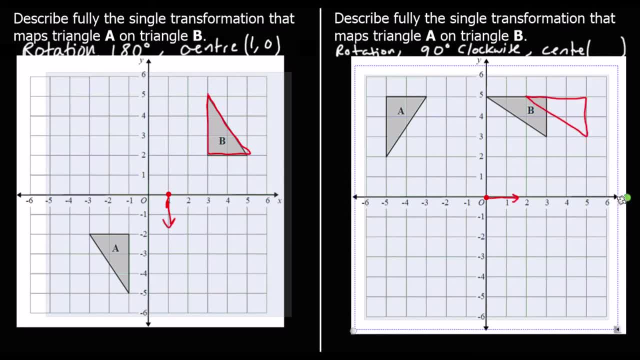 I'm gonna have to move it to the left so I could try holding the tracing paper at negative one zero. so move the shape, draw the shape. so with tracing paper you wouldn't have to move the shape, you could just hold the tracing paper in a different place. so let's give that one a. 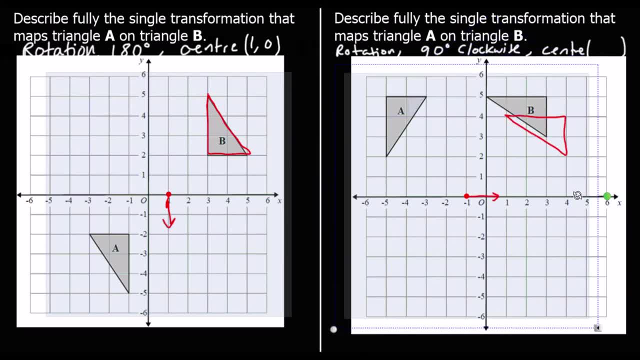 go, we rotate it, we can see it's in the wrong place again. so where else could we hold the tracing paper? if we try negative one one, we can see that works. so if we hold the tracing paper at negative one one, we can see that the tracing paper is in the wrong place. so we can see that the 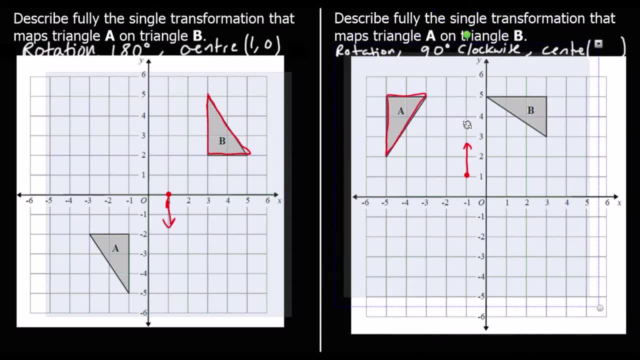 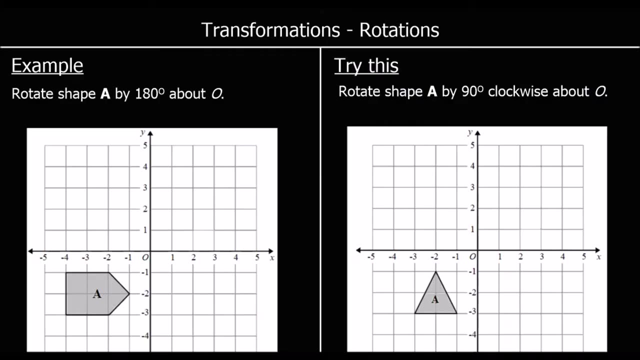 that shape A goes on to shape B, So our centre is at negative 1, 1.. Here we have a different question. This time we're being asked to rotate the shape. So it says: rotate shape A 180 degrees about the origin. So what we can do is we can get. 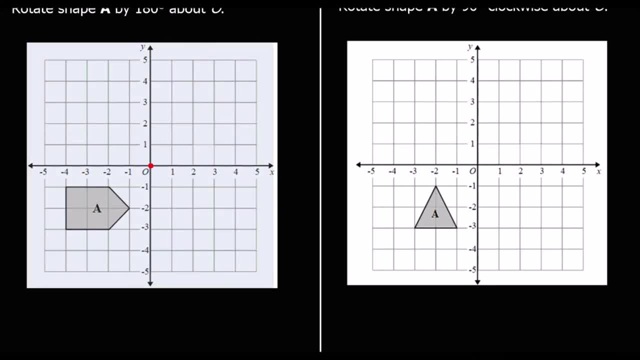 some tracing paper. We're going to hold our tracing paper at the origin. I'm going to draw a line going up, So I'm going to have to spin this line around 180 degrees, So it'll be going down when it's in the right place. I'm going to draw around the shape. 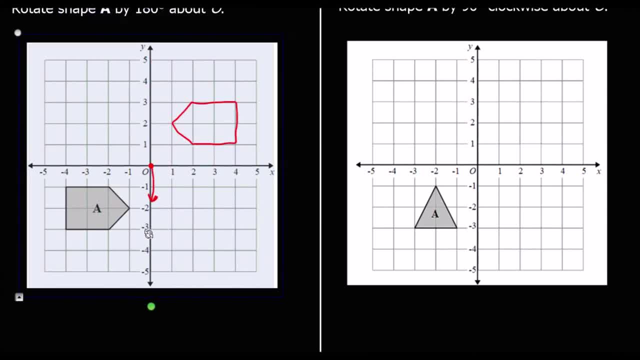 I'm going to rotate it 180 degrees. So that is where my shape has to end up. So this is where my shape has to end up. So if I draw the shape on and then take the tracing paper away, there is my transformed shape. 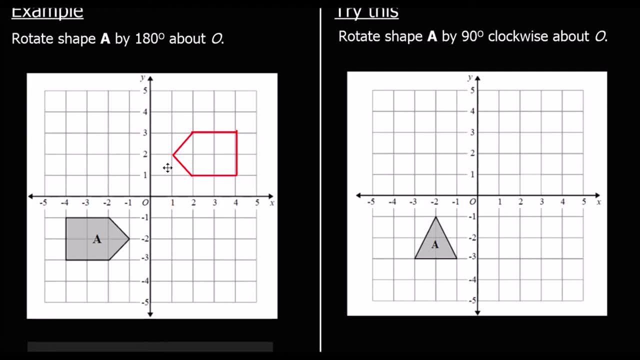 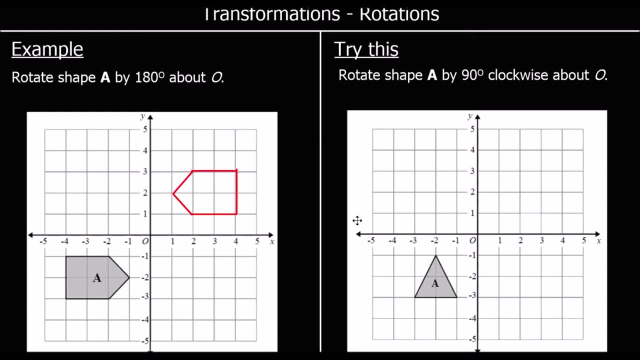 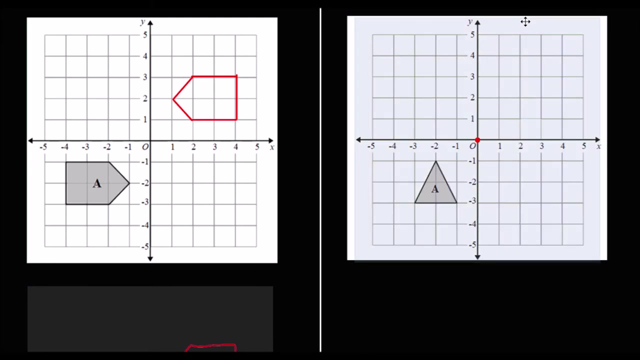 So that shape A rotated 180 degrees about the origin. Here's another question: Rotate shape A 90 degrees clockwise about the origin. So give this one a go. So we've got shape A. we're rotating 90 degrees about the origin, So we can use tracing paper. 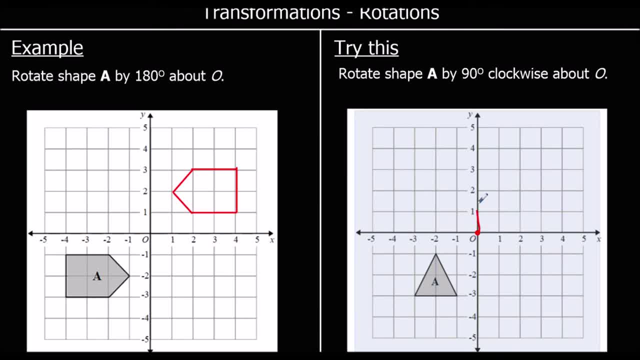 And we will have a line going up. We're moving this line 90 degrees clockwise, So it'll be going 90 degrees clockwise. So we're going to rotate 90 degrees about the origin, So we can move around 90 degrees clockwise. 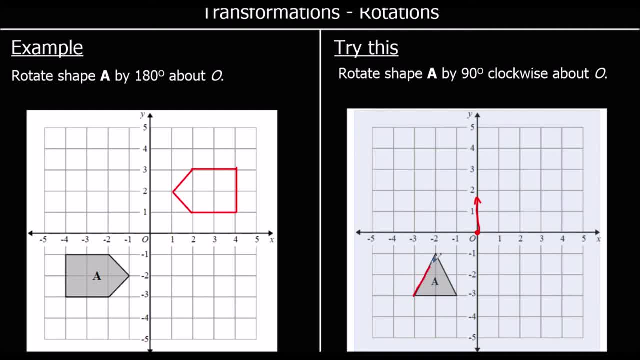 So it'll be on the x-axis, Then we'll draw around the shape. So we're going to rotate 90 degrees clockwise. So this is our new shape. So I'm going to draw, I'm going to draw the shape on, and then I'm going to take the back line here. 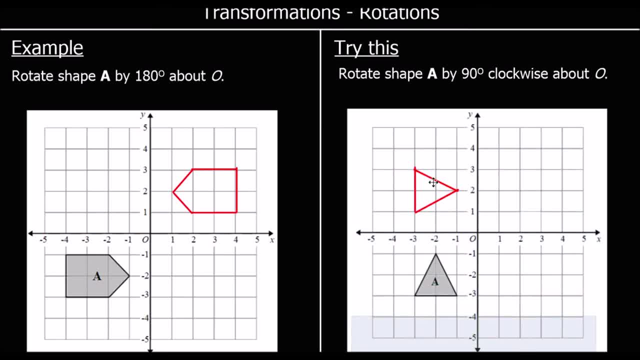 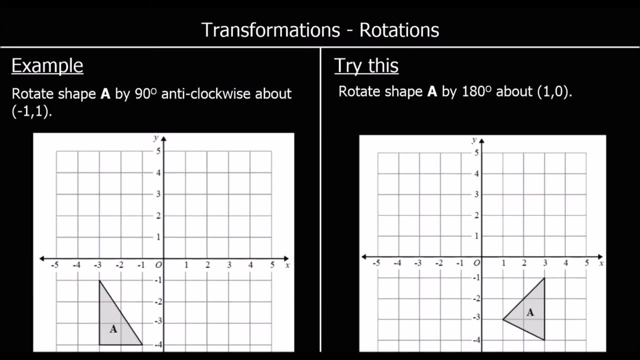 Because its ignored. So I'm going to take the back line here and then I'm going to take the front line here, the tracing paper away and there is our rotated shape. here's another one rotate shape: a 90 degrees anti-clockwise about negative 1: 1. so negative 1: 1, 90 degrees. 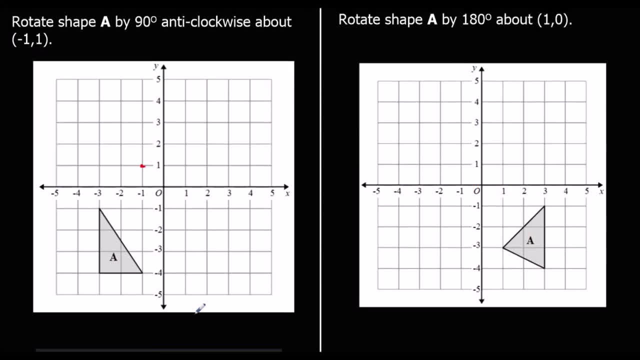 anti-clockwise. so we're going to be holding the tracing paper at negative 1, 1 and it's going to go 90 degrees anti-clockwise, so it's going to be facing this way. so, again, I'm going to draw around my shape, so I'm going to rotate it 90 degrees anti-clockwise, which is this direction. 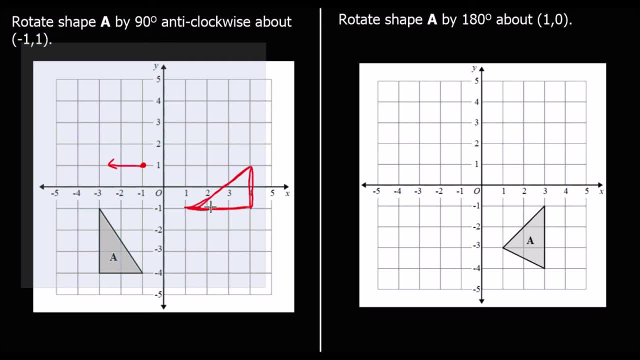 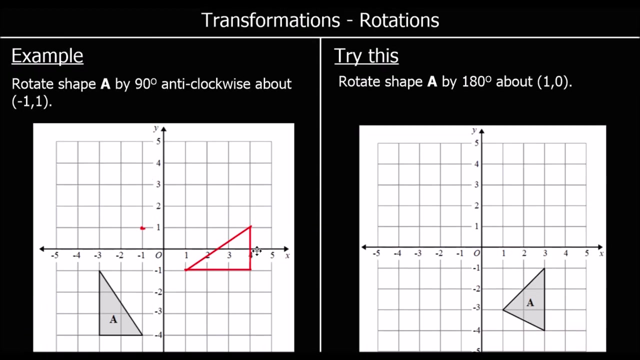 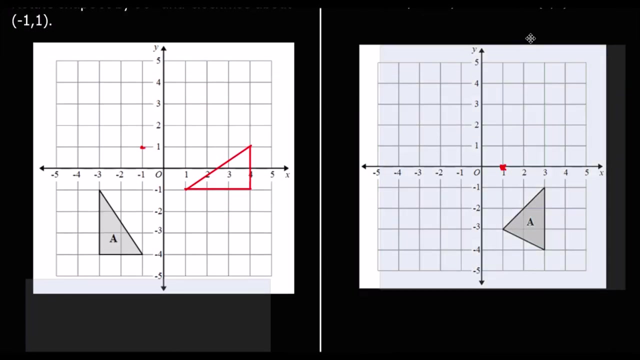 here's my new shape, and there is the rotated shape and one more 180 degrees about 1: 0. so 1: 0 is here rotating 180 degrees. so again, I'm going to use tracing paper. so I'm holding the tracing paper at 1: 0 and I'm going to rotate it 180 degrees. so this lines: 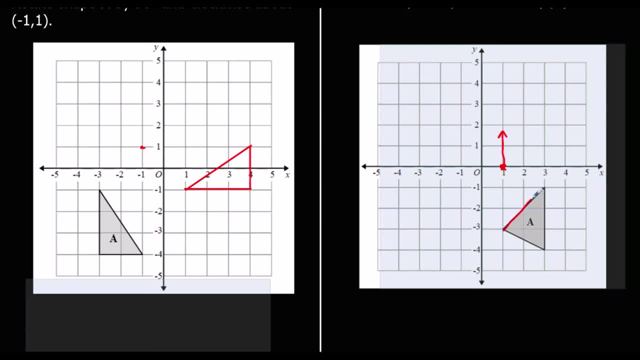 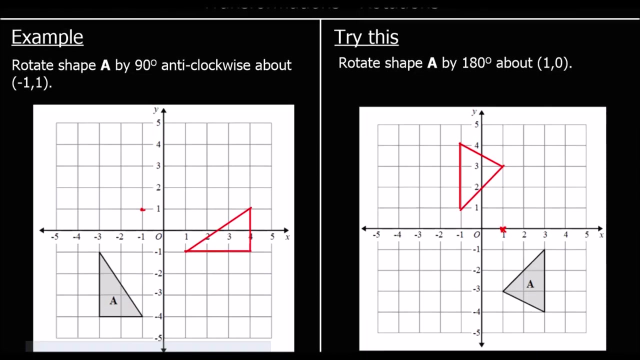 going up, it's going to end up going down. you rotate it 180 degrees. so there is my new shape. I'll draw around, draw the shape where the tracing paper has taken it to and take the tracing paper away, and there is the new shape. okay, two more questions, two questions to finish up. so 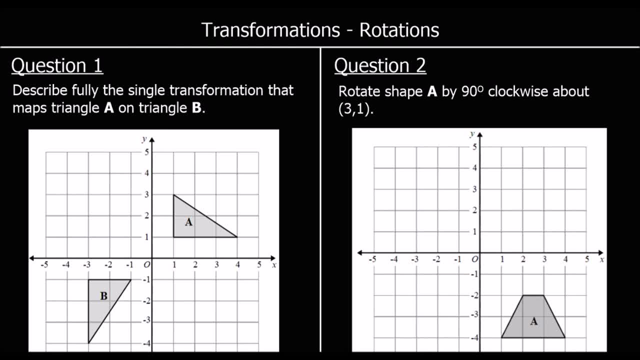 if you can pause the video and give these a go, do that? Add a new rule to all other本 cro49b. question one describe fully the single transformation that maps triangle a onto triangle B. so from looking at it we can see there is a rotation and it's gone. 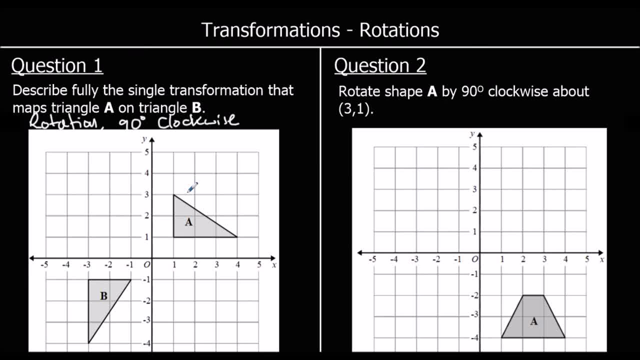 90 degrees clockwise and we need to know the centre. So where would we have to hold the tracing paper? So it's going to be around here somewhere. So it's going to be, say, three away from the middle, three away from the middle. 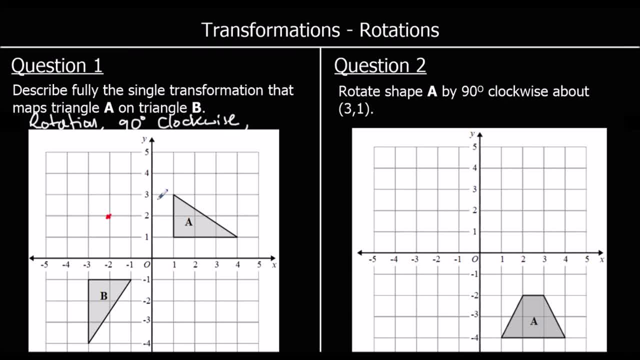 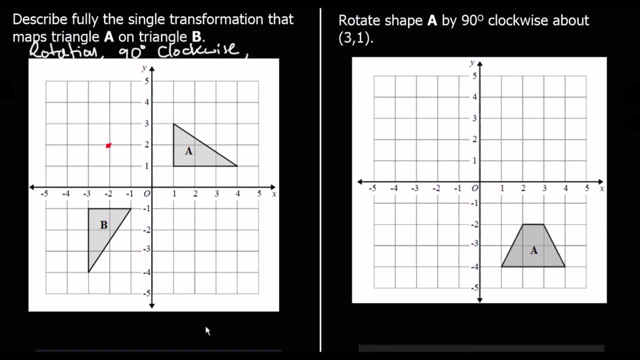 Across one up one across three across one down three. So it's going to be here and I'll use tracing paper to check that. So that's going to be where I hold the tracing paper, at the centre. It's going to be 90 degrees clockwise. 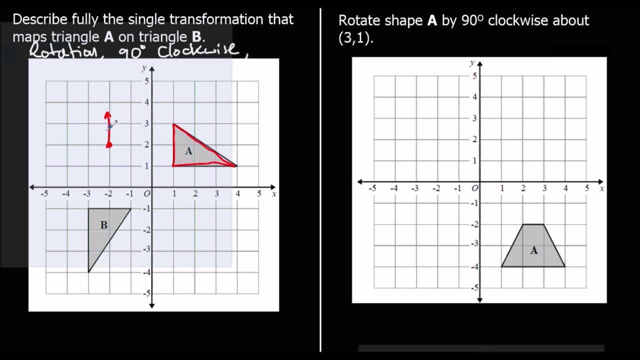 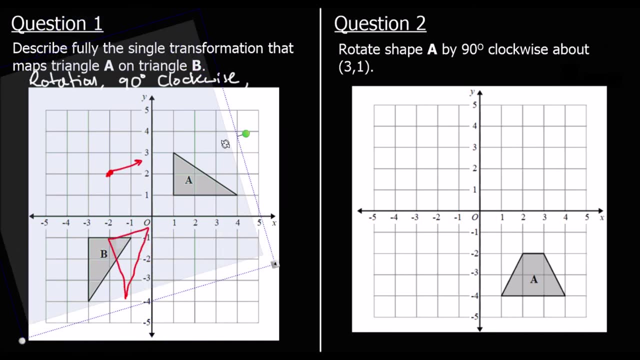 So it's going to be a turn to the well, 90 degrees clockwise, so a turn, a quarter turn to the right. So I'm going to turn it 90 degrees clockwise. so the arrow is going to the right and there is shape B. 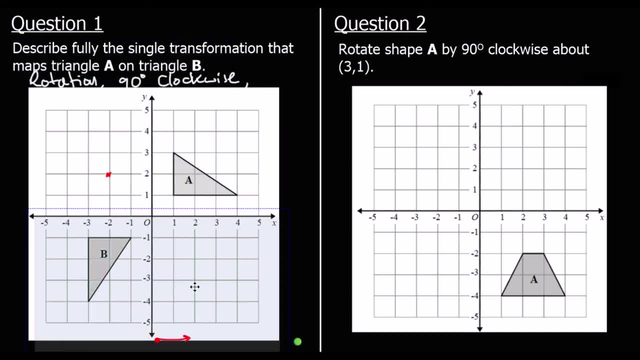 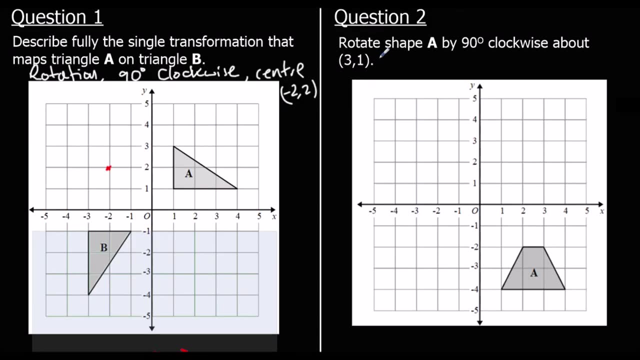 So that is a centre at negative 2, 2.. And question two: rotate shape A 90 degrees clockwise about 3, 1.. So 3, 1 is here, So it's going to go 90 degrees clockwise. 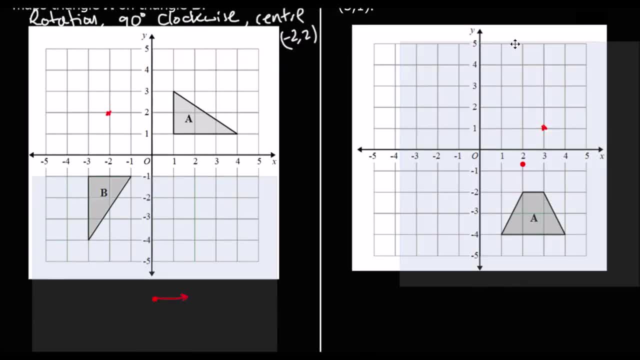 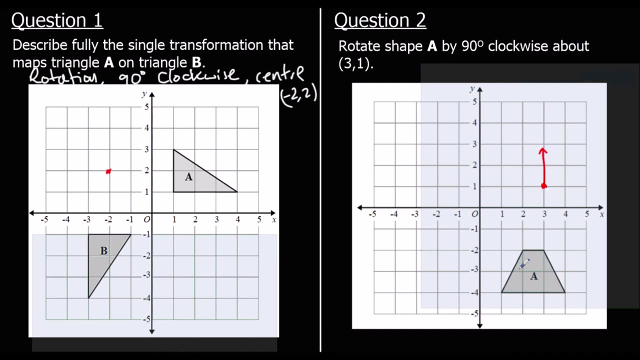 We can use tracing paper, So I'll get the tracing paper at the centre at 3, 1.. That's why I'm going to hold the tracing paper when I rotate it. So the line's going up at the moment. If it goes 90 degrees clockwise, it'll be going to the right.